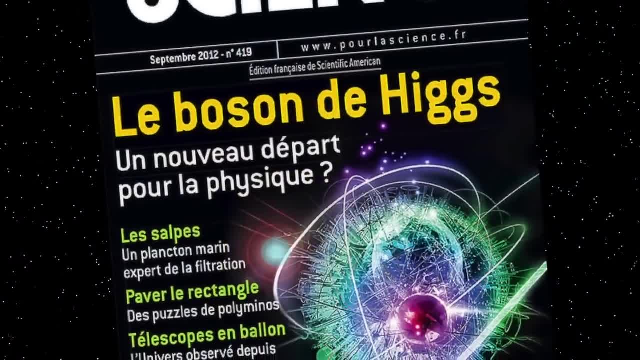 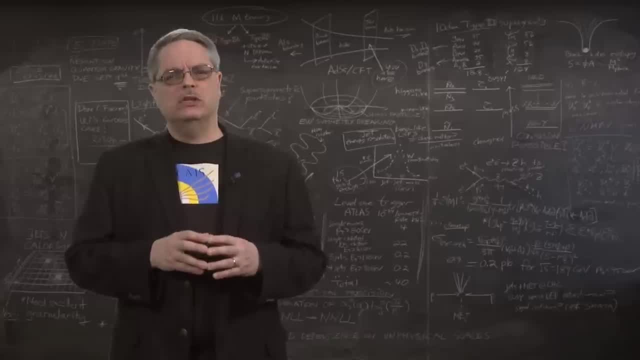 This particle, which was the last unconfirmed prediction of the Standard Model of particle physics, and an accomplishment that took nearly half a century to achieve. If you're watching this video, you've almost certainly heard reporters say things like: LHC: scientists discover the Higgs boson. 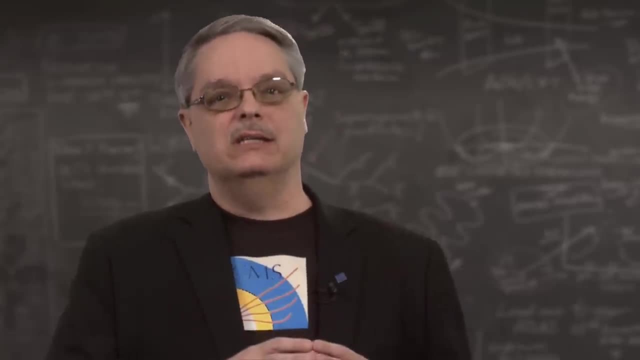 However, even as amazing as the LHC is, it's not the entire story. Being able to accelerate particles with the LHC is a crucial capability, but until you can record the outcome of the collisions, you really aren't doing the science that the accelerator was built to. 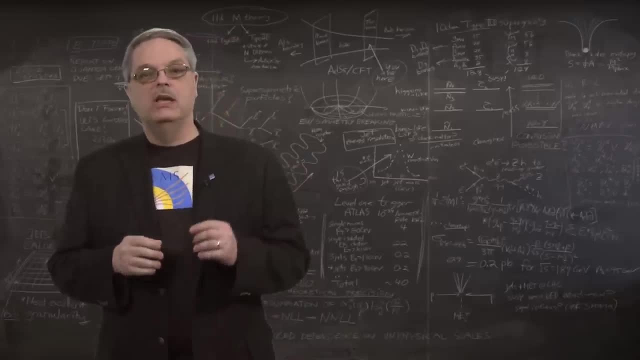 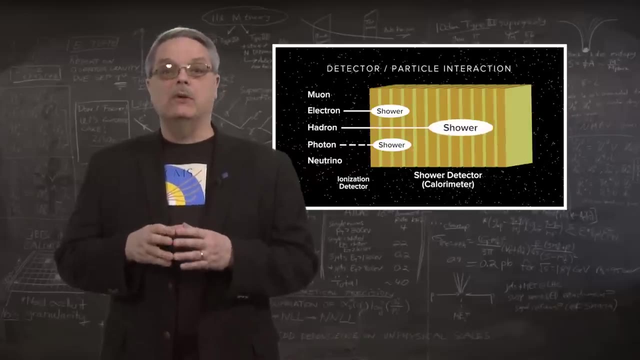 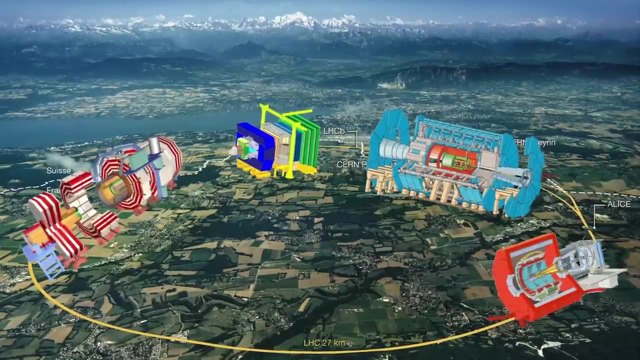 do To capture these collisions, you need to use particle detectors. I made an earlier video about how particle detectors work, but in this video I want to talk about the specific detectors at the LHC. There are four main detectors at the LHC, each with unique capabilities. Each one is 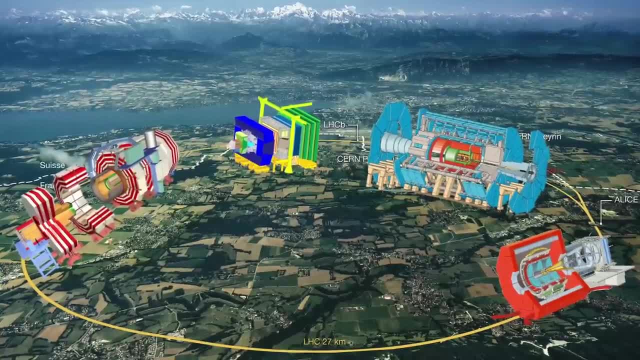 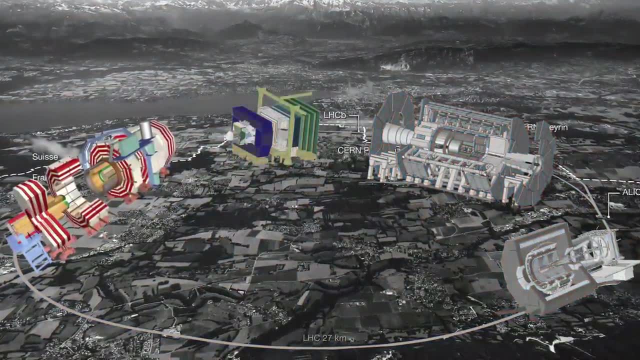 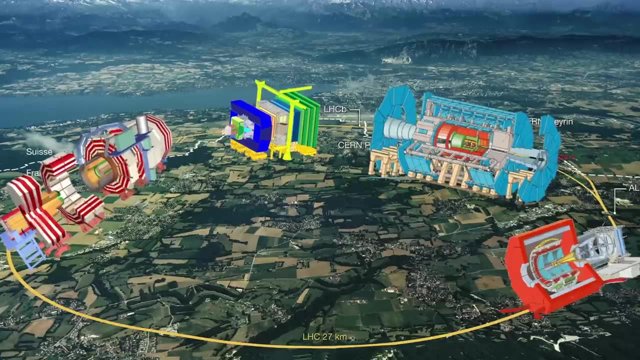 basically a huge camera that can study millions or billions of particle collisions per second. The four detectors are called ALIS, ATLAS, CMS and LHCb. ATLAS and CMS are the ones involved in the discovery of the Higgs boson, while the other two are specialty detectors. 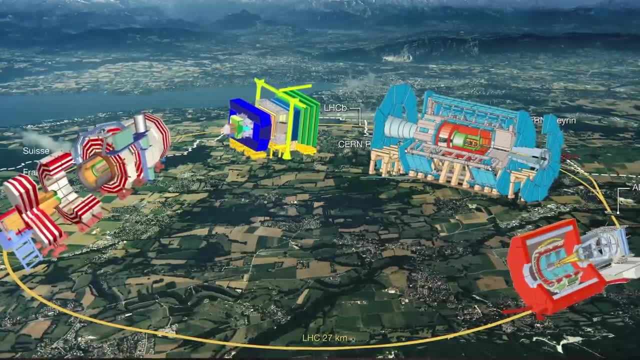 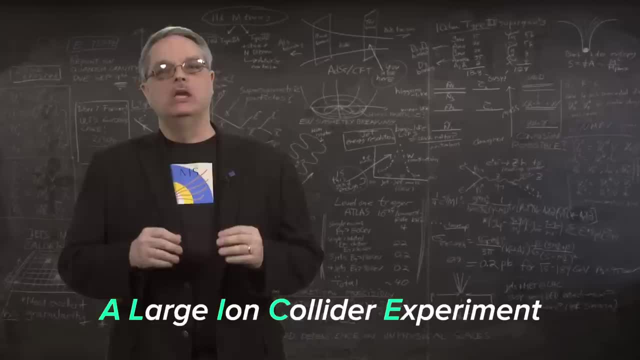 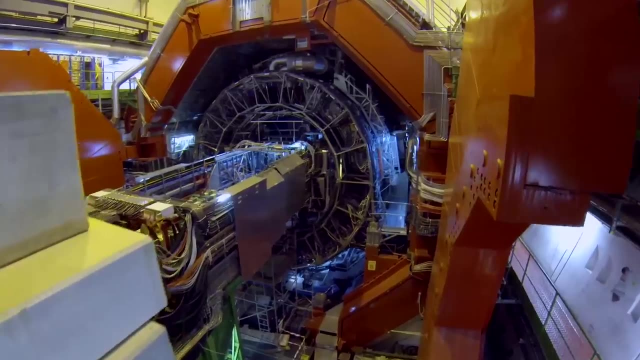 So let me tell you a little bit about each one in turn. ALIS, sometimes pronounced Elise, stands for a Large Ion Collider Experiment and is designed to study what happens when you collide two nuclei of lead together. It is 26 meters long and 16 meters high and weighs 10,000 tons. It takes about 1,500 physicists from. 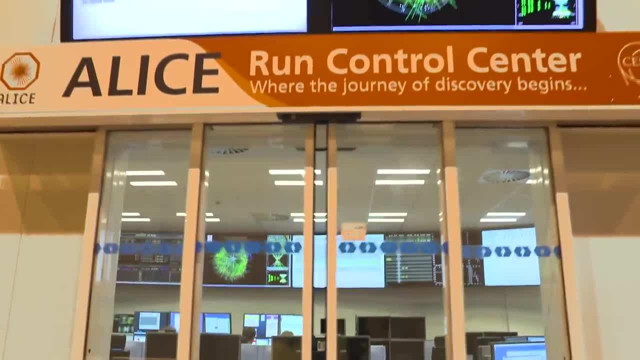 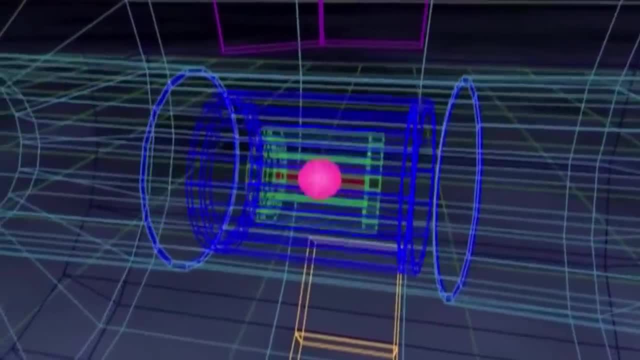 154 institutes in 37 countries to perform. Its purpose is to study a new state of matter called a quark-gluon plasma, in which matter is heated to a hundred thousand times hotter than the center of the sun, hot enough to literally melt protons and neutrons at the 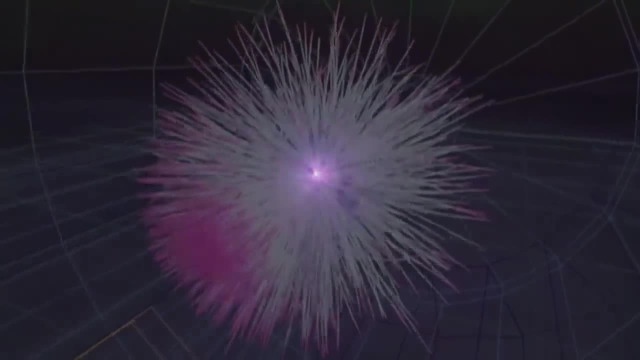 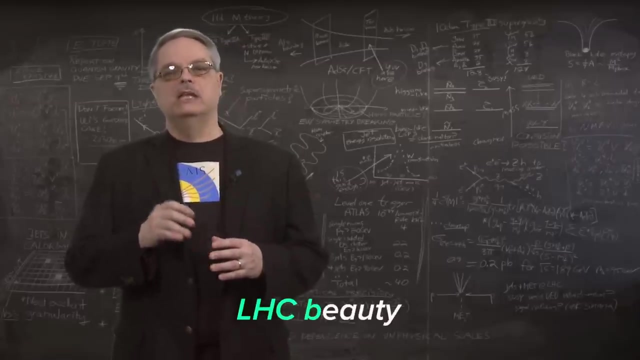 center of atoms. Conditions like these were last common in the universe about a millionth of a second after the Big Bang. The LHCb experiment is quite different. Its core purpose is to understand why the universe is made of 100% matter, when our best understanding of the early moments of the universe say that. 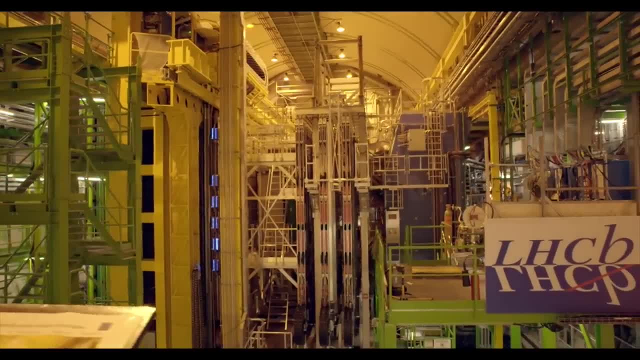 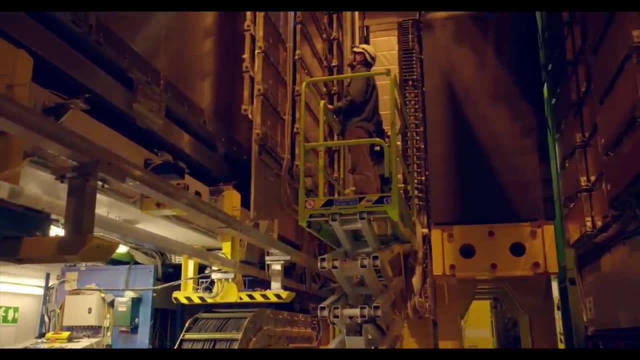 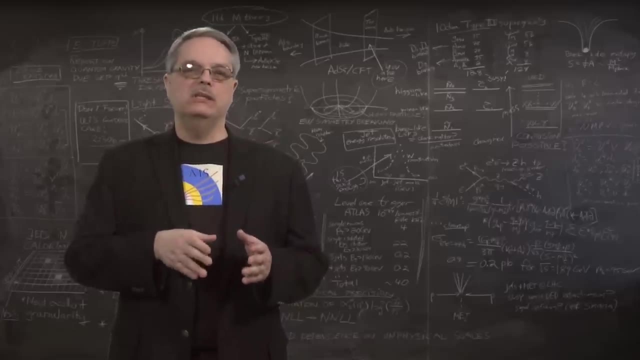 matter and antimatter were made in equal quantities. It weighs about 4,500 tons. about 700 scientists representing 69 universities and laboratories from 17 countries are involved. The name LHCb means LHC beauty, as beauty is an older name of a heavy and unstable quark. 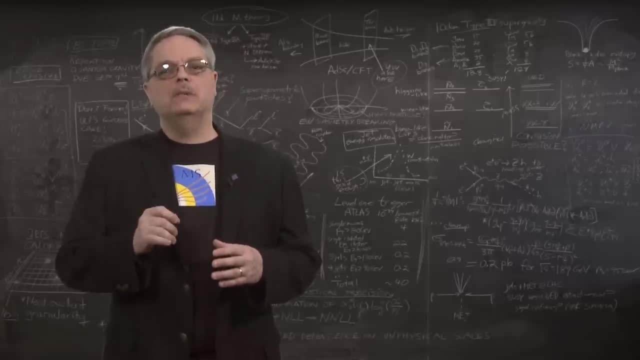 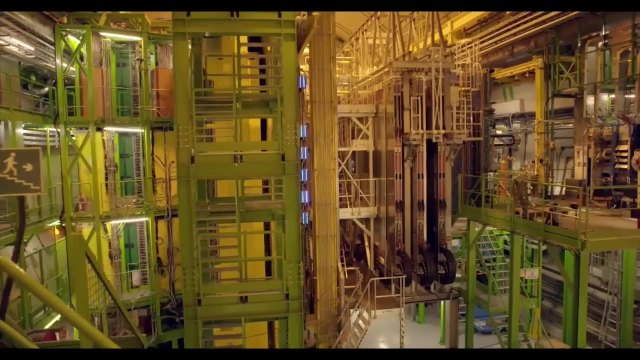 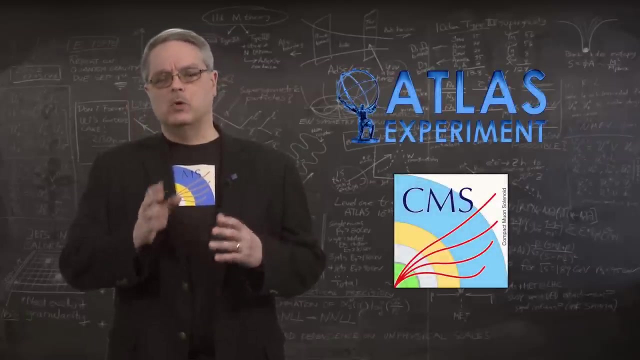 While that name is well beautiful, it is now more commonly called the bottom quark. It is thought that studying this ephemeral particle is the most promising way to shed light on this puzzling asymmetry between matter and antimatter. The ATLAS and CMS experiments are more similar in their fundamental goal. These two detectors 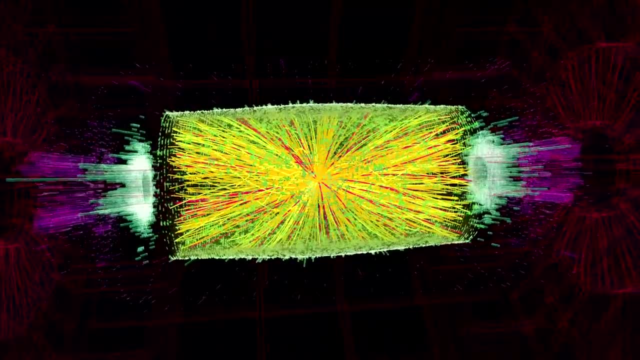 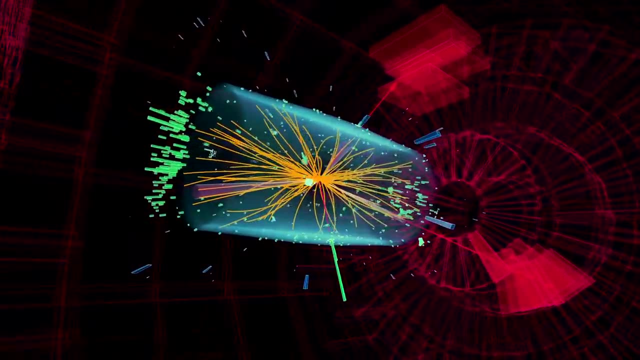 are designed to record collisions between beams of protons at a collision energy of 14 trillion electron volts. The energy densities in these collisions haven't been common, since the universe was less than a trillionth of a second. old Collisions occur at a rate. 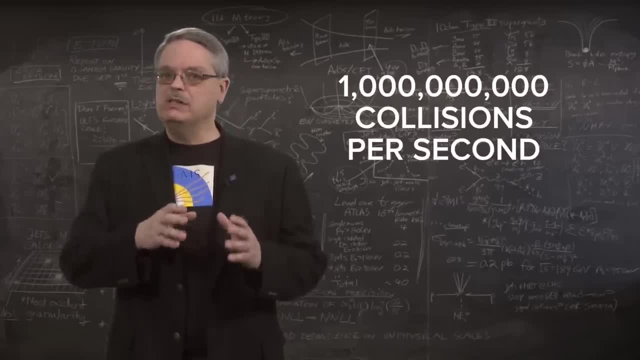 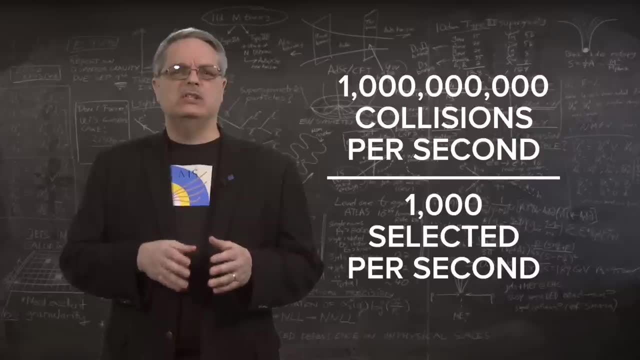 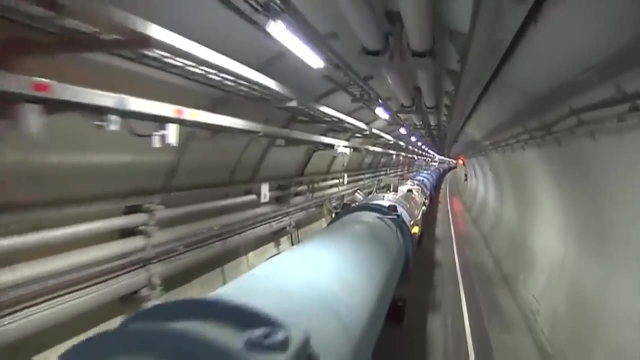 of a billion times a second, and these detectors inspect every single collision before recording only about a thousand select collisions each second. You may have heard that the LHC is colliding beams at 13 trillion electron volts, but that's just to ensure that we can run the accelerator reliably. It also means that if 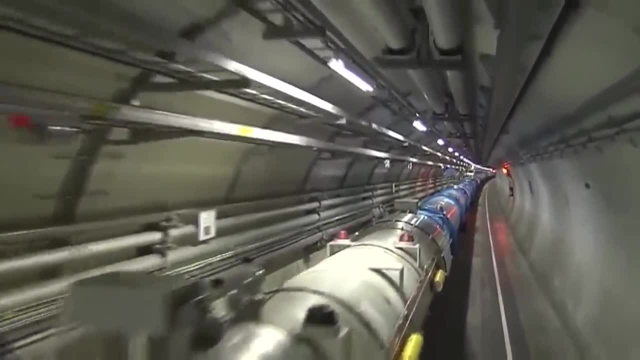 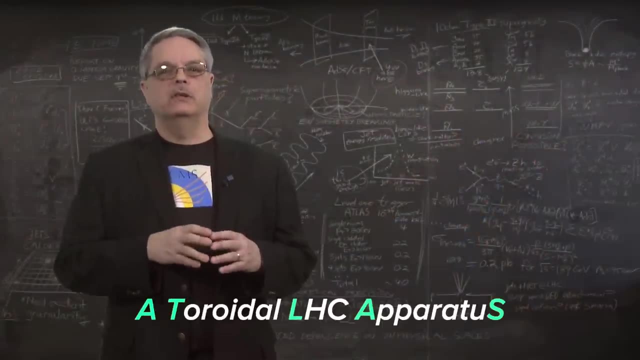 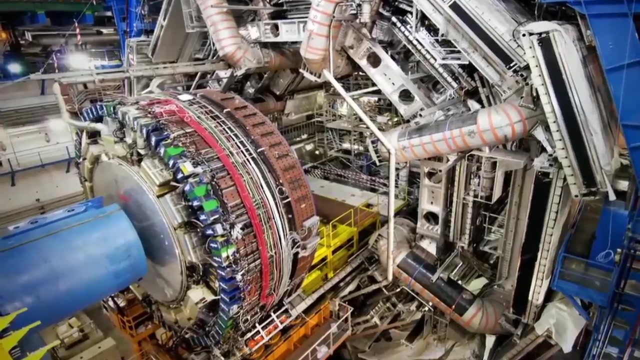 we have more experience with a machine, we might still squeeze out another 7% or so more energy. The ATLAS experiment is physically the largest particle experiment ever built. Its name is an acronym for a toroidal LHC apparatus. It is 45 meters long, more than 25 meters high. 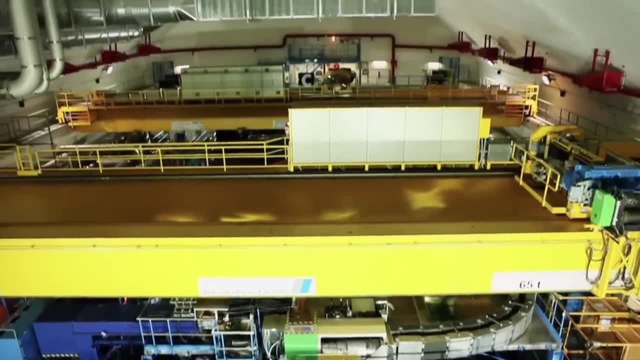 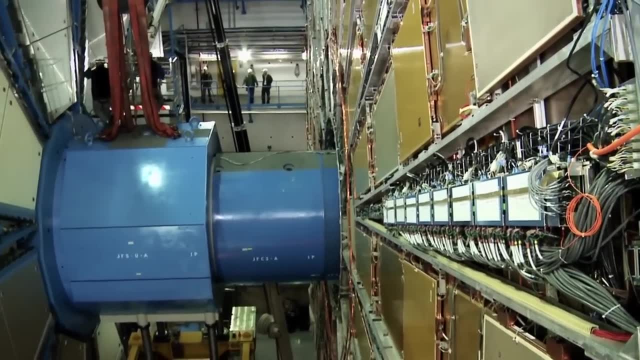 and weighs about 7,000 tons. The LHCb is the largest particle experiment ever built. It's about half as big as the Notre Dame Cathedral in Paris and it weighs the same as the Eiffel Tower. It involves over 3,000 scientists from about 180 universities and laboratories from 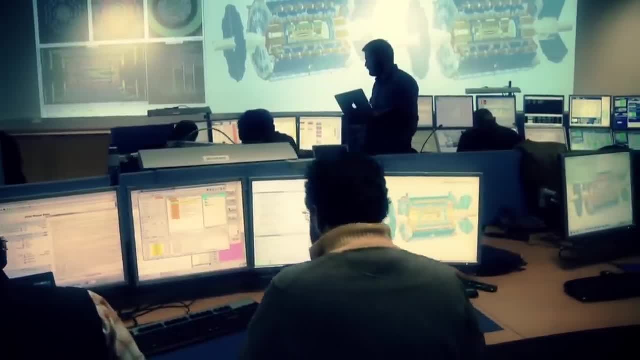 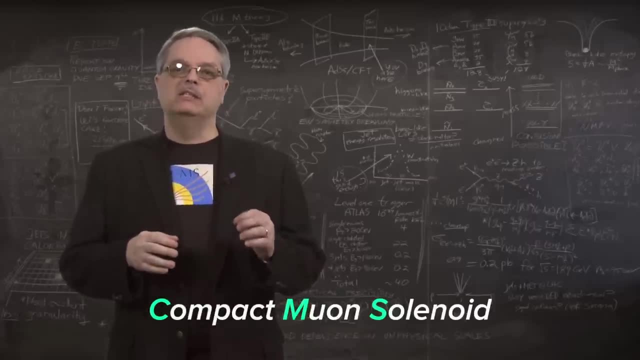 38 countries. More than a thousand PhD students do their research using this detector. The Compact Nuance-Ellenoid Experiment, or CMS, has some significant commonalities with ATLAS, but looks different in detail. For one thing, it is more massive, weighing 14,000. 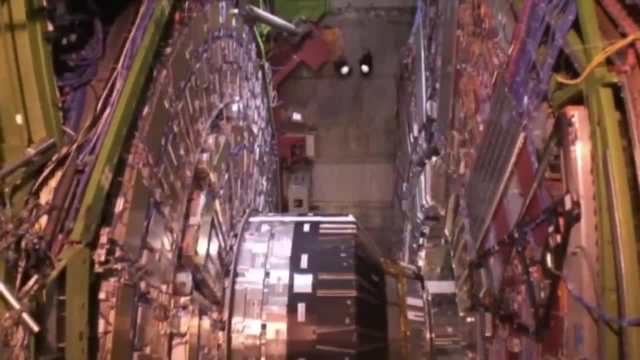 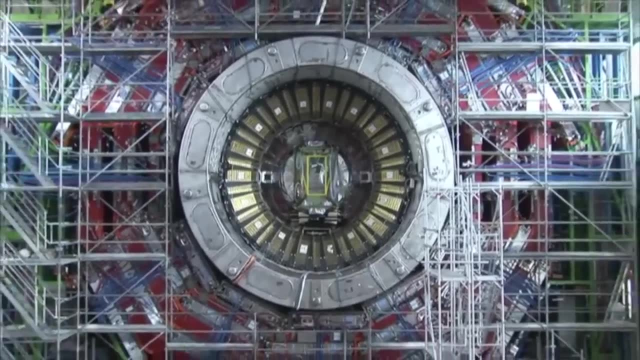 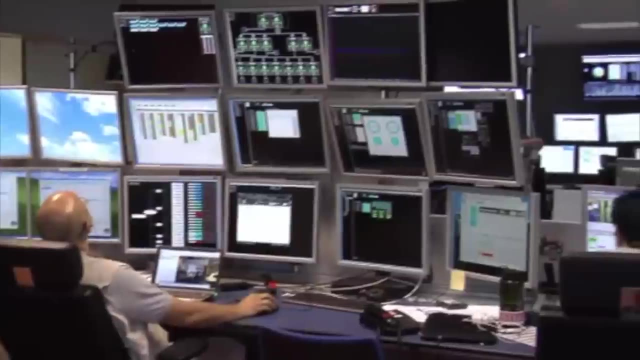 tons, or about twice the weight of the Eiffel Tower. It is 22 meters long and about 15 meters in diameter. The detector consists of about 100 million individual elements. Like ATLAS, CMS requires 3,000 scientists to design, build and operate from 182 institutions.